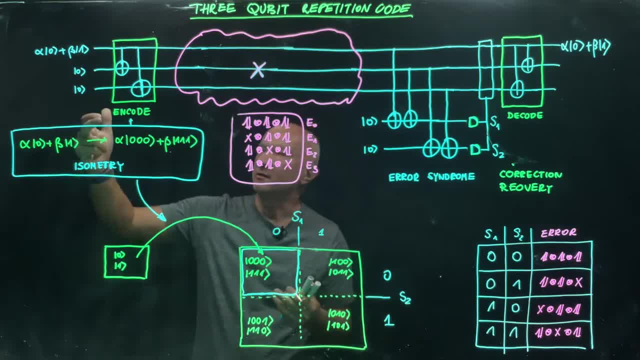 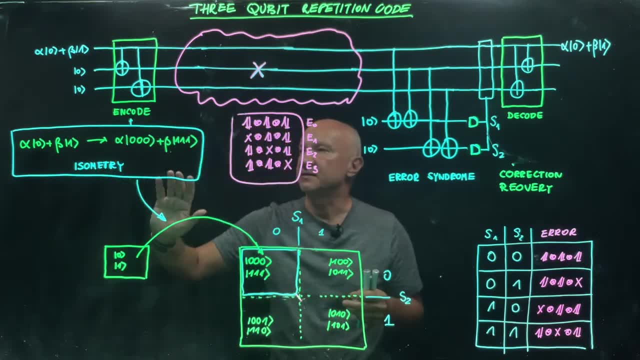 a unitary operation, so that your original state, in this case alpha zero plus beta one, is embedded in a dimensional Hilbert space and it becomes a highly entangled state of three qubits: alpha zero, zero, zero plus beta, one, one one. So, as you can see, you can recognize now. 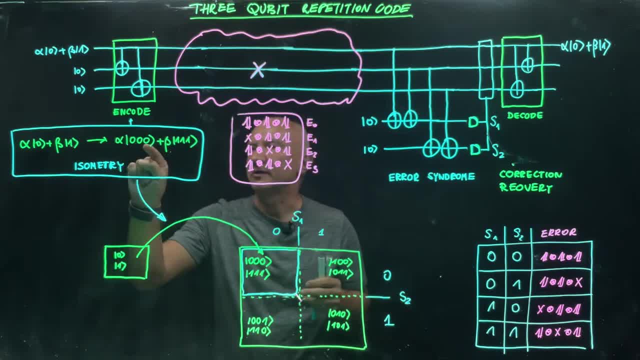 what we will call the code words. So zero in the original qubit will become vector zero, zero, zero in the encoded space and one will become one one one. So think about it this way. So I have two dimensional Hilbert space associated with my state, and now I'm just going to insert this two dimensional Hilbert space. 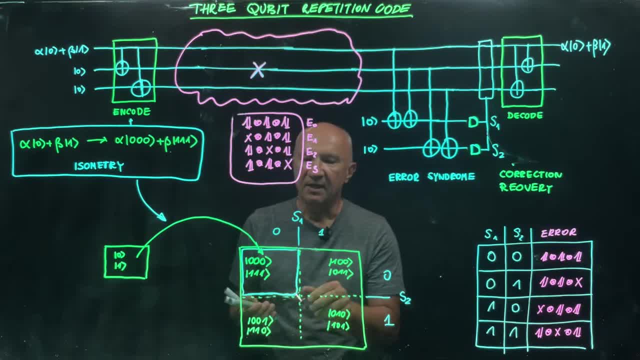 into eight dimensional Hilbert space, So it becomes a coding subspace. So at this point, now we are after this operation, when we are here, your mathematical sort of intuition should see a dimensional Hilbert space, and in that a dimensional Hilbert space you have two dimensional coding. 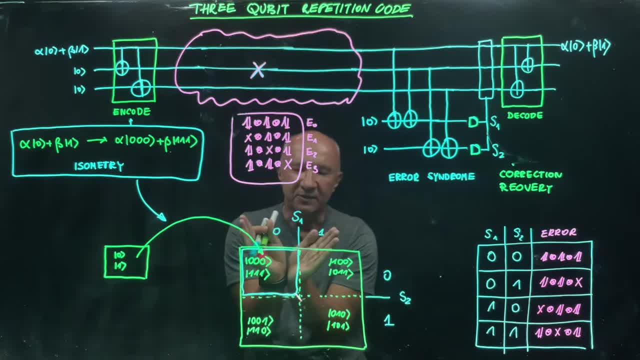 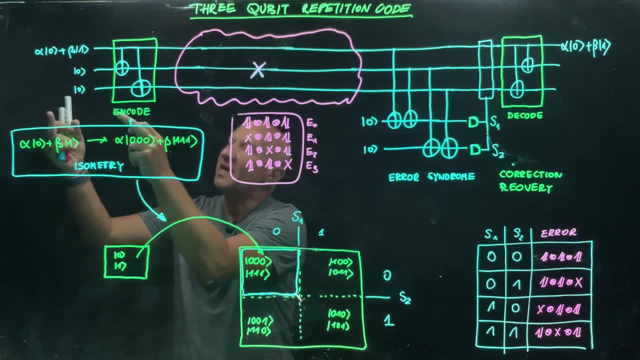 space which is spanned by two qubits of space, basis vectors 0, 0, 0 and 1, 1, 1, and some unknown vector, psi, which is of the form alpha 0 plus beta 1 is. is there in, in, in that state, in that subspace? here it. 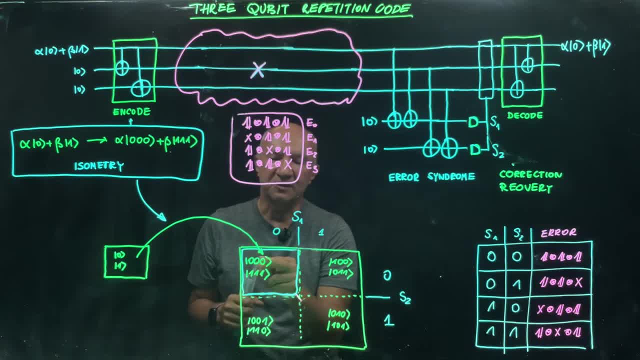 becomes alpha 0, 0, 0 plus beta 1, 1, 1. so we call it encoded version of of this state. now errors happen, so we are moving now to the second segment. we have three qubits here and the four things can happen. so we of course we assume that we. 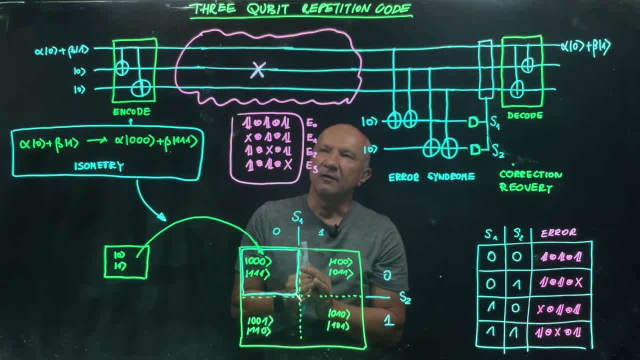 assume that there is a completely positive map, which is defined by the four Krauss operators, or four errors. so the one is that no error happens. so that's, that's the situation where nothing happens to our three qubits. then e 1 is describes the error on the bit flip error on the first qubit. e to the 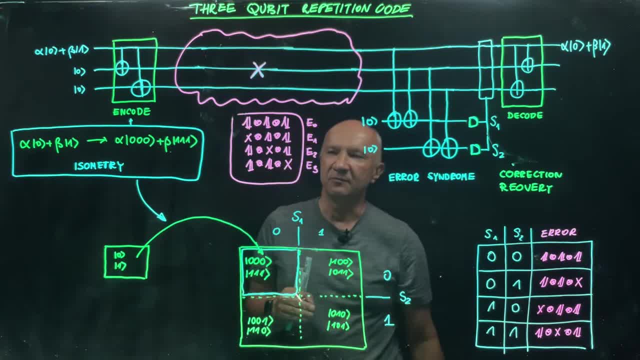 bit flip error on the second qubit and e 3. as you can see, the bit flip error on the third qubit. now let's let's take a look how those errors modify the code subspace. so, as you can see, e0 of course doesn't do anything to the code subspace, so that's fine. the the whole subspace is. 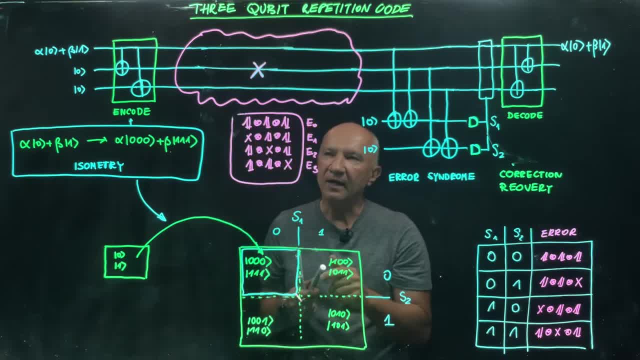 is intact. but then e1, which is a bit flip on the first qubit, takes the whole code subspace and moves it to an orthogonal subspace which is spun by vectors 1, 0, 0, 0, 1, 1. right, so we just apply the bit flip to the to the first. 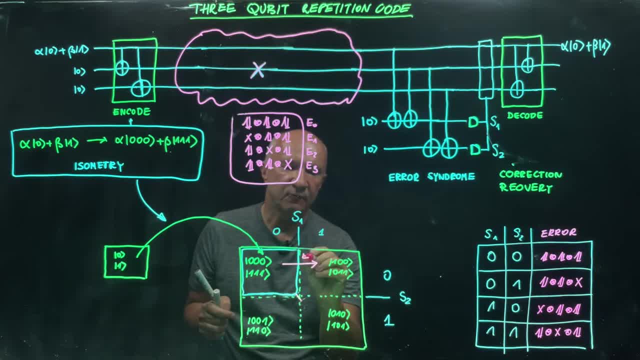 qubit. so you can see that the result of e1 is shifting the whole subspace without modifying, without you know doing anything. it's a nice unitary operation which, when you're, when you sort of restrict it to the input being this being vectors from the code space, the whole code spaces and shifted to the other. 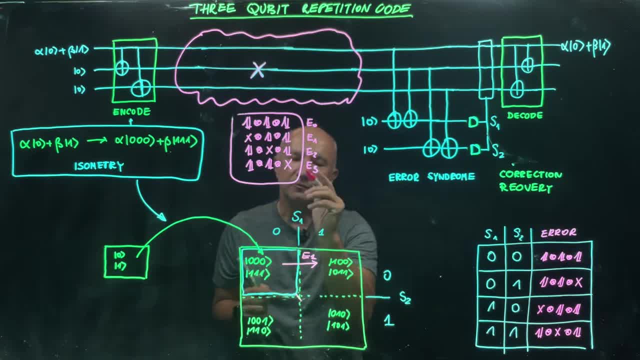 which is orthogonal to it. then e tool does a similar job. it just takes the whole code subspace and generates and shifts it into an orthogonal subspace which is spun by vector 0, 1, 0, 1, 0, 1. and e3 does a similar job, right? so, as you can, 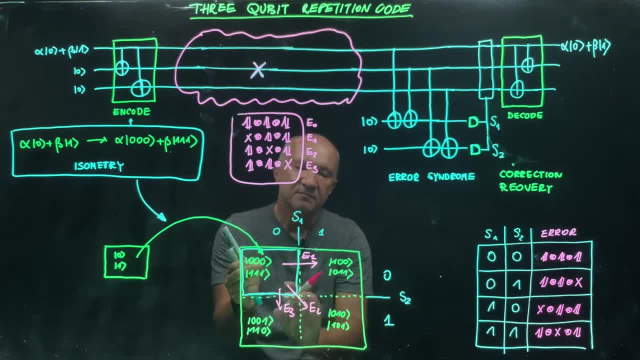 see that we have three non-trivial errors here, and each of them takes the original code space into a subspace, which is called an error subspace, which is- and all of them are mutually orthogonal. so, in principle, you can distinguish where is your state at this point. right, because we can perform the measurement that will allow us to. 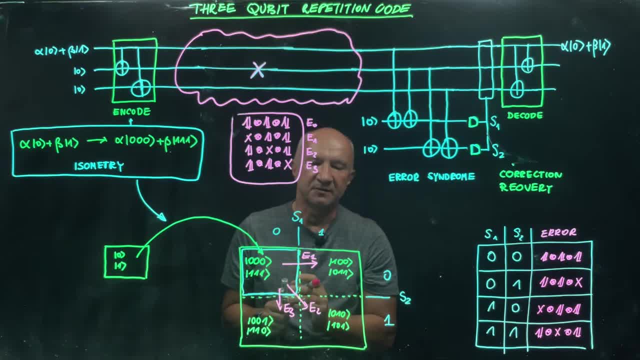 differentiate between those different orthogonal subspaces. we want to figure out at this point which error happened, and we would like, once we know it, we can reverse the whole operation right. so if you just somehow figure out that it was e tool that happened, then you can just simply. 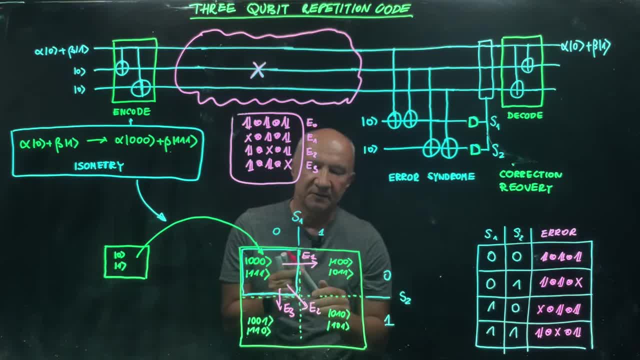 apply again the bit, flip to the second qubit and you just reverse this arrow and you're back into the coding space and in order to find out which error happened, then, indeed, we perform the measurements. in fact, we perform the two measurements: one and that will differentiate between those two. 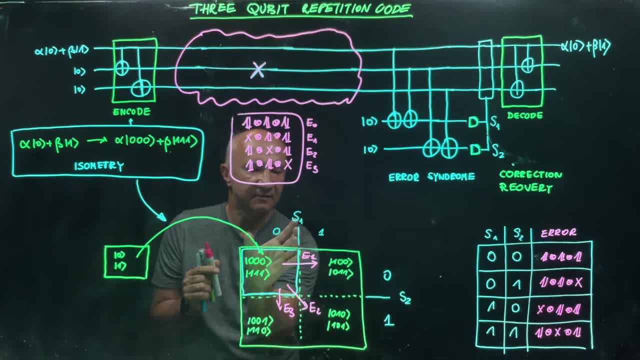 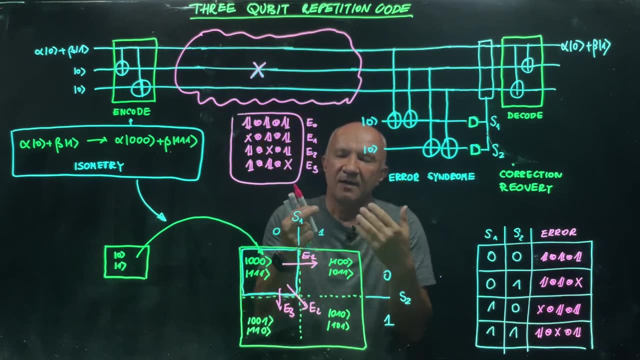 subspaces. so we look at the two four dimensional subspaces and the other measurement that will just differentiate between those two subspaces. so let me just show you how we implement this measurement. this is this called like error syndrome: finding out which particular error happened, that the 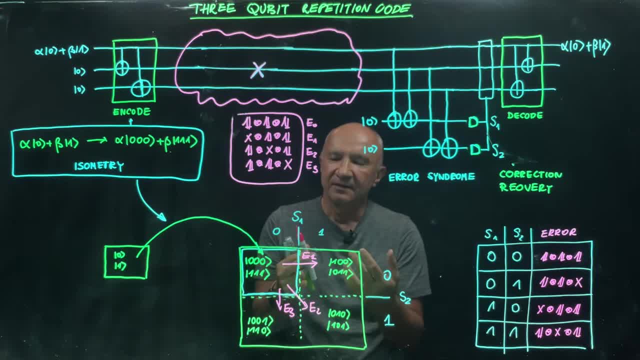 you call this is a error syndrome. you'll find out what actually happened in the system and the measurement, the, the first one, which can distinguish between the subspace where the bit values in the basis states on the first two qubits are identical or not identical, is constructed by the two control. 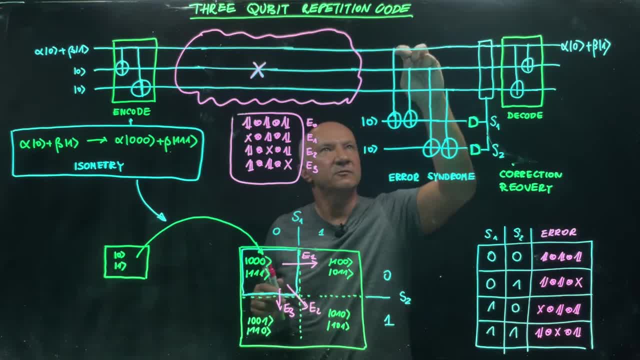 notegates acting on auxiliary qubits. so what you do? you just simply take the first two qubits as your control qubits. you then take a target qubit, initially in state 0, you apply two control notegates and, if you see the outcome, 0. 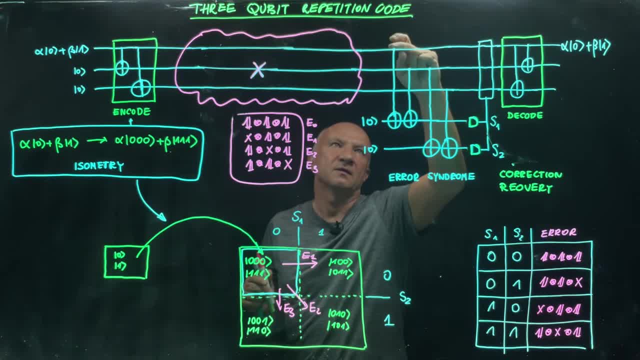 that means either those two qubits are in state 0- 0 or in state 1- 1, in which case you know you flipped the target qubit twice. so in other words, whenever you see zero as the outcome of one, we call here S1 measurement. that means that the the entries in the base. 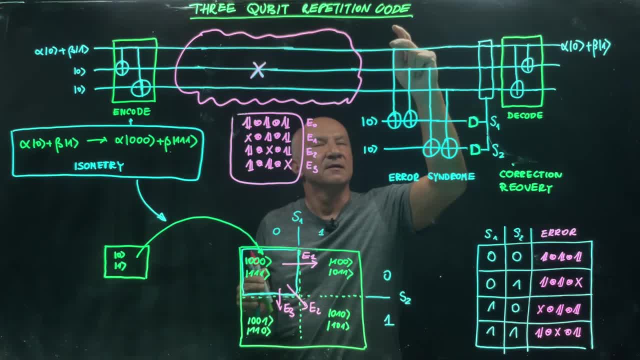 state, so that the state here is identical, either 0, 0 or 1, 1, and you know, of course the 3rd qubit could be anything. so this particular measurement here projects on the subspace, which is spawned by 0, 0, 0, 1, 1, 1. 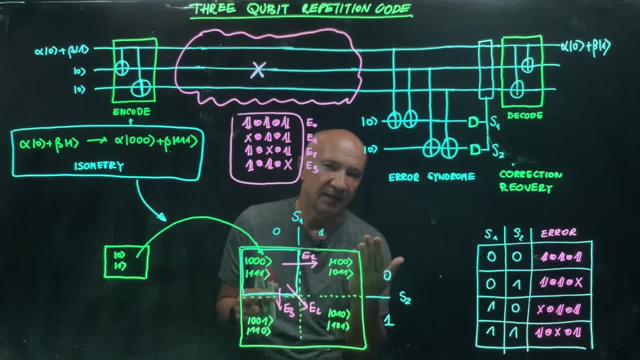 0, 0, 1, 1, 1 0 and the orthogonal subspace. So by performing this measurement, you can distinguish between whether are you here or are you here Like is your state located somewhere on this side or on this side? and by the same token, by the same line of argument, you check the 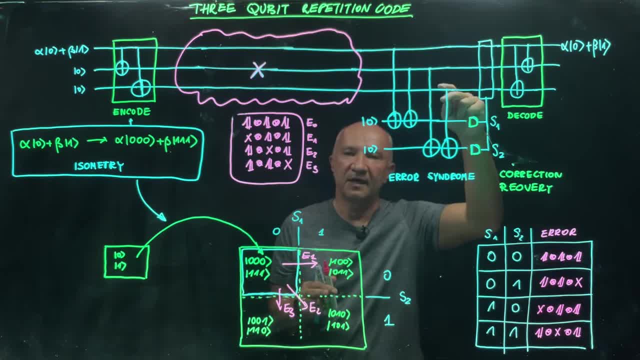 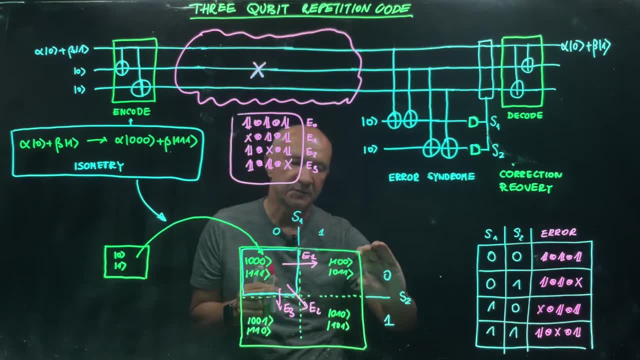 parity of the second and third qubit and then you can just figure out whether are you in this subspace, here in this four-dimensional subspace, or are you in this four-dimensional subspace. So suppose the error happened in the second qubit, so you have a bit flip on the second qubit. 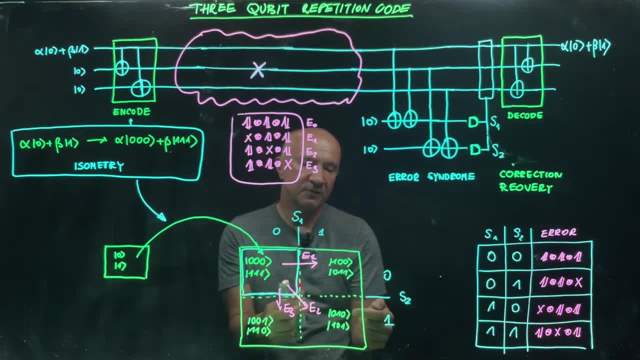 So in which case we are here, so you can see in which case the S1 measurement will give you the value 1, because you are located in the subspace here, and S2 will also give you 1.. So you can see that, knowing the two outcomes, 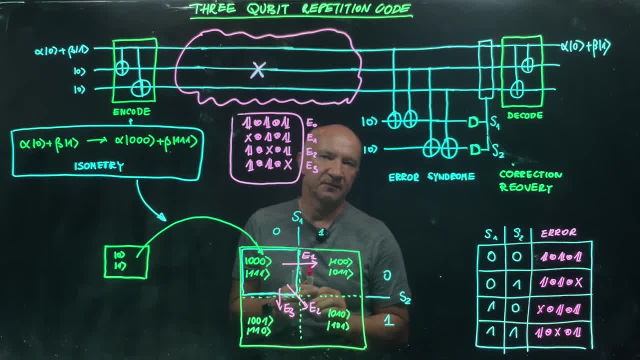 you can identify in which subspace is your state, So you can identify which particular error happened, So we can construct a very simple lookup table. So when we when two outcomes are 0- 0, so we have S1 is equal to 0 and S2 is equal to 0. 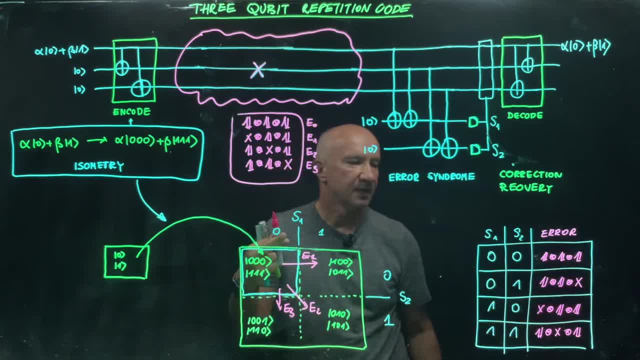 then nothing happened. You are sitting in this subspace here, And then, for example, if S1 is equal to 1 and S2 is equal to 0, so S1 is equal to 1, S2 is equal to 0, then you know that the first qubit was affected. 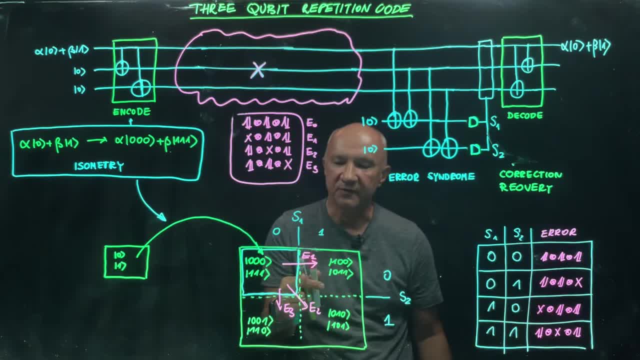 So that's the case here. So you had a bit flip on the first qubit. So this gives you the error syndrome, the value of S1, S2, and from the error syndrome you can figure out what actually happened in the system And then that allows you to correct the error. 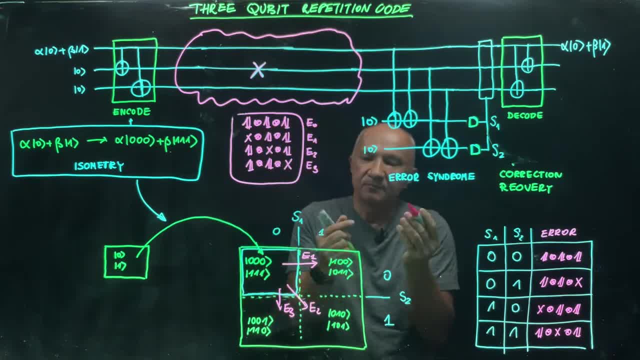 So at this point you simply read the the syndrome and reset the state to the original value, to the back to the coding space, So you shift the error subspace back into the code subspace. Then, once this is done, of course, then you just decode the state which is like: 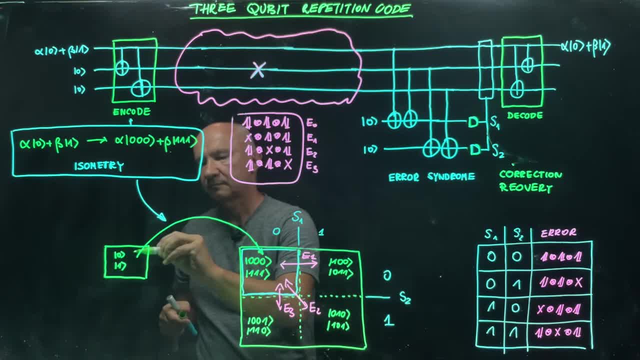 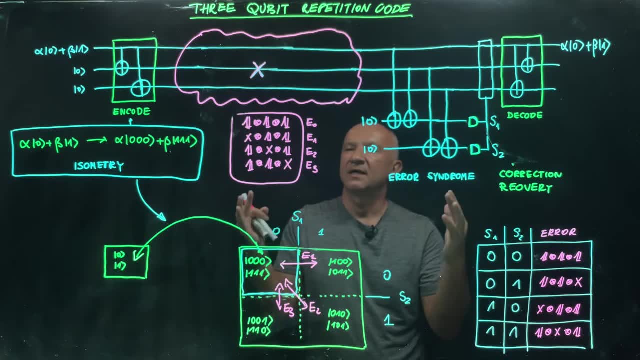 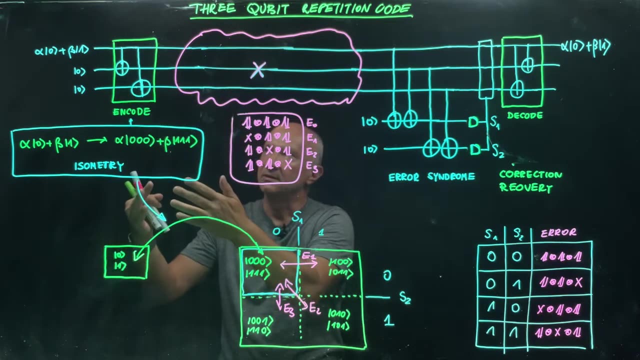 reverse of this operation and you go back into your original state. So this is how how it works. You have encoding. I hope you see how unknown quantum state can then be mapped into a state in higher dimensional Hilbert space, So the whole two-dimensional Hilbert space associated with the original qubit. 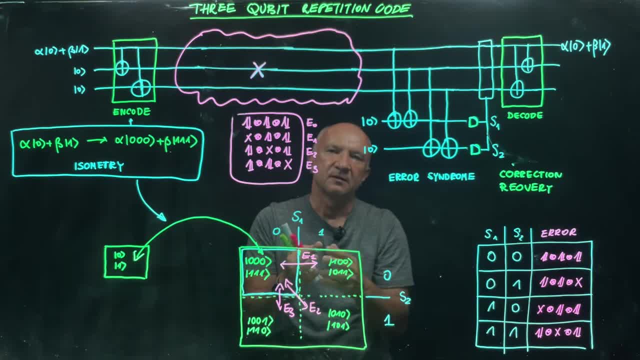 becomes two-dimensional code space in some higher dimensional Hilbert space, And the good thing is now that the state is spread over a number of qubits. In this case, the state of one qubit is spread over three qubits, So that means that if anything happens to one particular qubit, we have this redundancy. 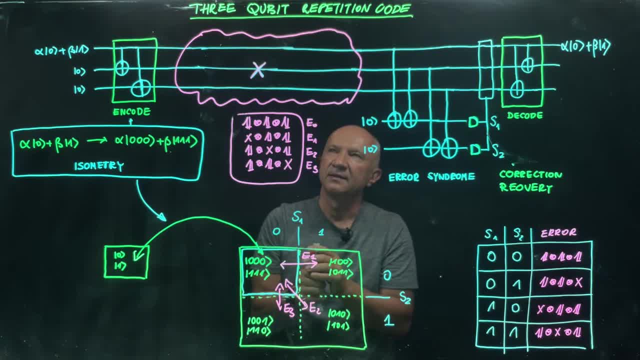 We can figure out what happens And try to reset it. And then, as you can see, we have. we assume of course here a rather artificial, completely positive map, But you know, we have to start somewhere. We have to show that we can deal at least with bit flip errors. 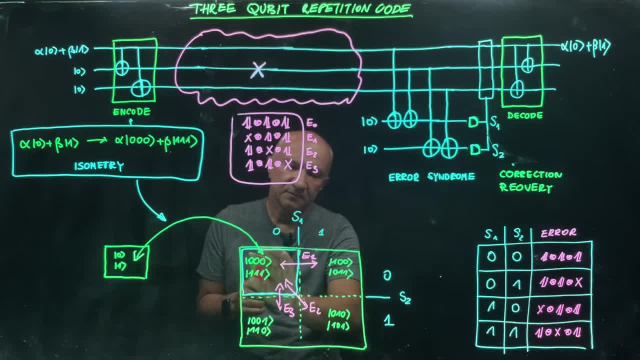 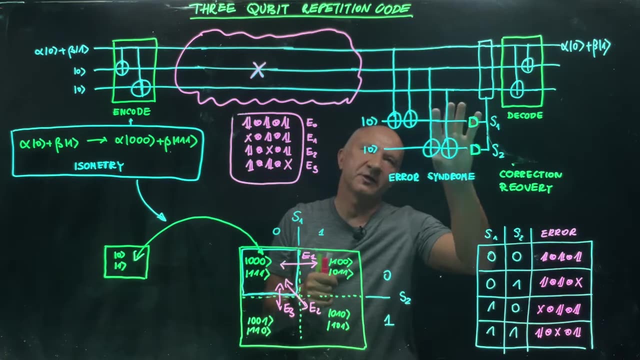 And we can see that those errors actually shift the coding space into mutually orthogonal subspaces. So once we can figure out what happened, we can really just reset the whole thing, And we, just in order to find out what happened, we we bring ancillary qubits. In this case, we just bring two more qubits and we 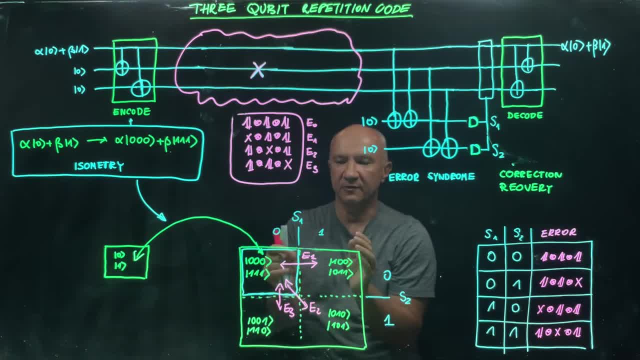 perform those measurements. But those measurements are gentle kind of measurements, right? So they they sort of differentiate between the subspaces. So you search: where is your state? Which particular subspace is your state residing, The one that after the error, By bisecting, 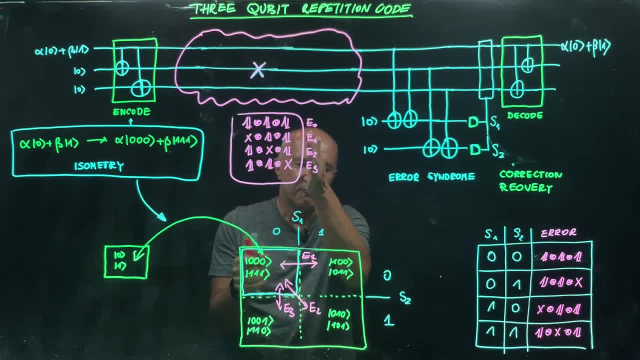 your Hilbert space, this higher dimensional Hilbert space. So first you you look at the result of the S1 measurement, which somehow bisects the Hilbert space into those two four dimensional subspaces. So now you know whether it's on this side or on this side. 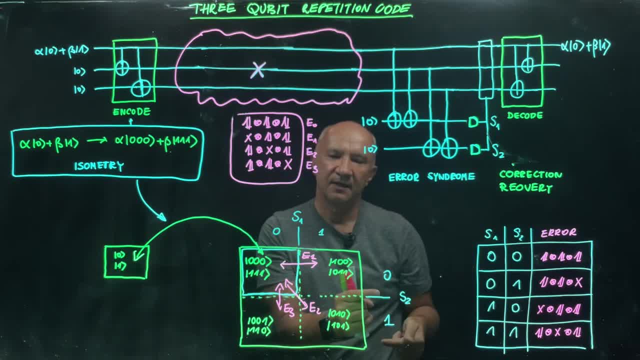 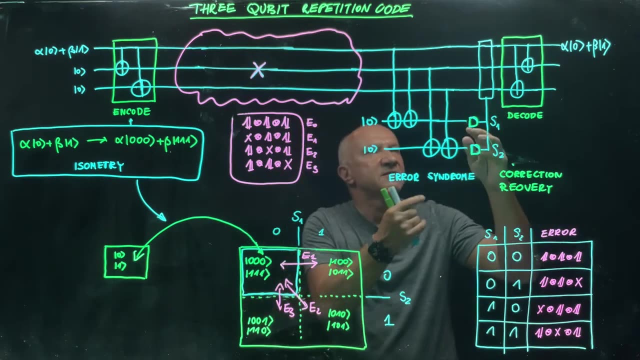 And then you have S2 measurement, which is another error syndrome, which tells you: are you on this side or this side? So this is just another bisection of the Hilbert space, And then you just do the corrections. By the way, even though I said you measure, it doesn't have to be. 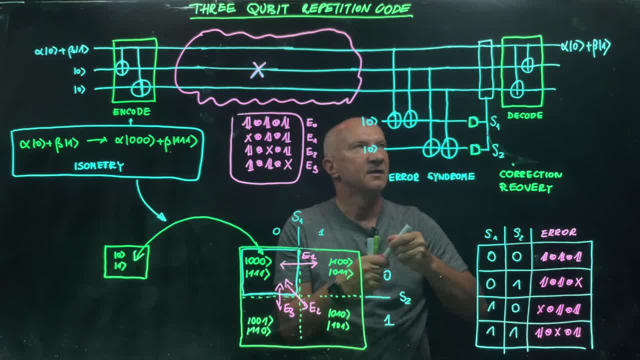 the measurement per se. You can have a unitary operation here which is conditional unitary of some sort, where basically it says, okay, if 00, then do nothing, If 01 then apply this unitary. So you see it, somehow somehow controlled unitary operation. 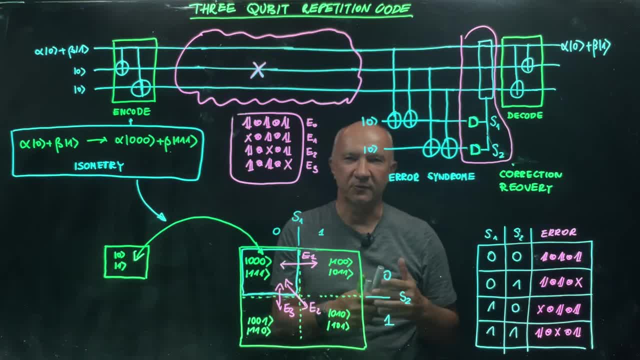 So that could be done by one big unitary operation. It doesn't have to be a measurement per se, But if you prefer to think about the measurement, that's also fine. And then, once you reset the whole thing to the original code space, the decoding gets you back to.